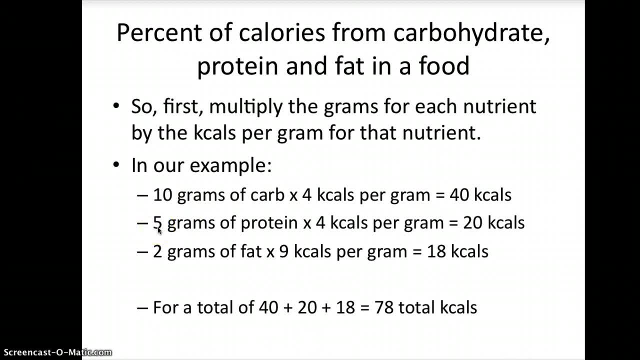 Protein. in our example we had 5 grams of protein. We know that there are 4 calories per gram of protein. So 5 grams times 4 calories equals 20 calories. Same for fat: 2 grams of fat times 9 calories per gram for 18 calories. 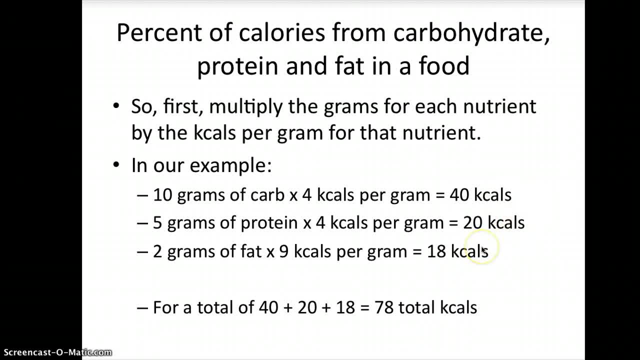 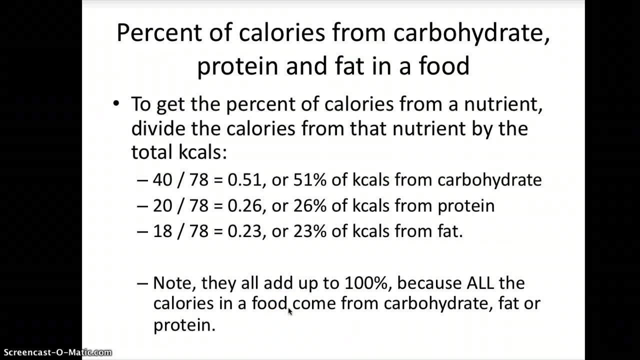 Now these are All the calories from the different nutrients. You add them up to get the total calories. So 40 plus 20 plus 18 equals 78 total calories. The last step is to get the percent of calories from carbohydrate. Let's go back and look at the first step. 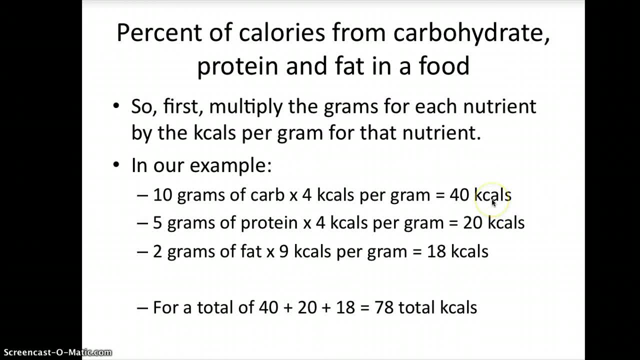 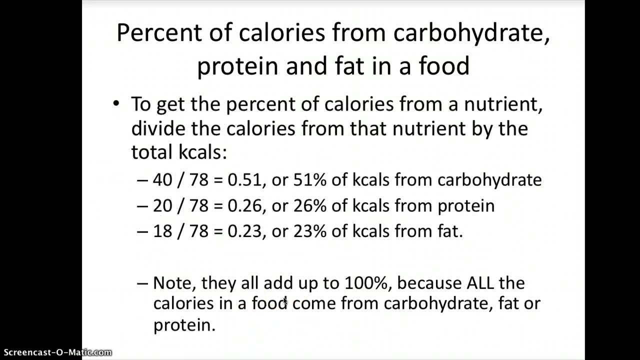 We were just figuring out the total number of calories from each of those nutrients. But what this number doesn't show us is what, What portion of the total calories, comes from that nutrient. That's what the next step is: Determining the percent of calories from that nutrient. 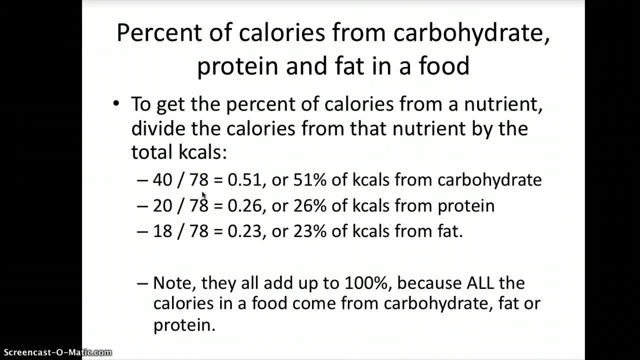 So if 40 out of the 78 total calories come from carbohydrate, that's equal to about 51 percent of the calories are coming from carbohydrate. So you would do 40 divided by 78. That equals. In your calculator you'll see 0.51. 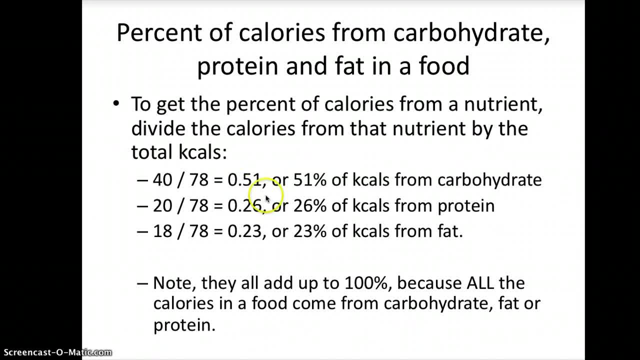 You can multiply. You can multiply times 100, or in your head you can just say that equals 51%. I lost my cursor, I'm sorry. Hold on, Let's see if- Ah, there it is. In your head, you can say that equals 51%. 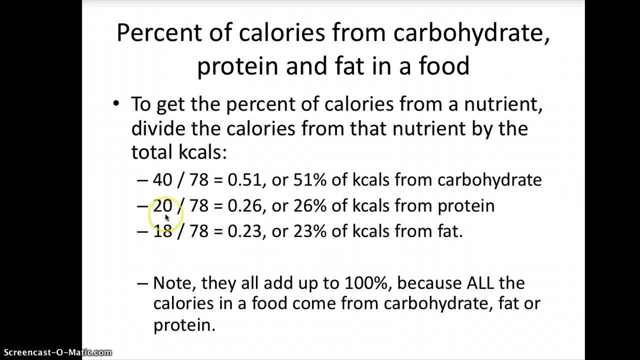 Okay, same for the protein. You would take the calories from protein, compare it to the total number of calories. So 20 out of 78 equals about 0.26, or 26% of the calories come from fat. So 20 divided by 78.. 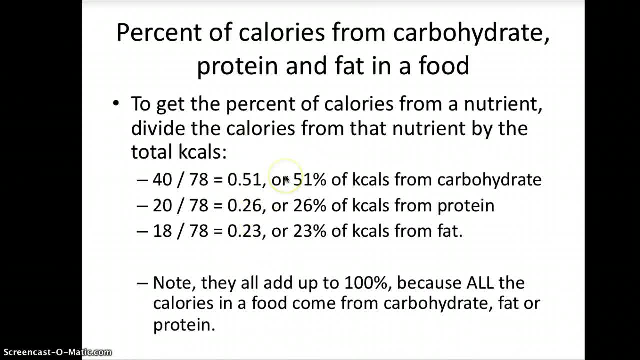 And lastly, for the fat same thing: 18 calories came from fat out of the total. So 18 divided by 78 is about 23% of the calories from fat. Notice that they all add up to 100, because all of the calories in a food come from carbohydrate, fat or protein.